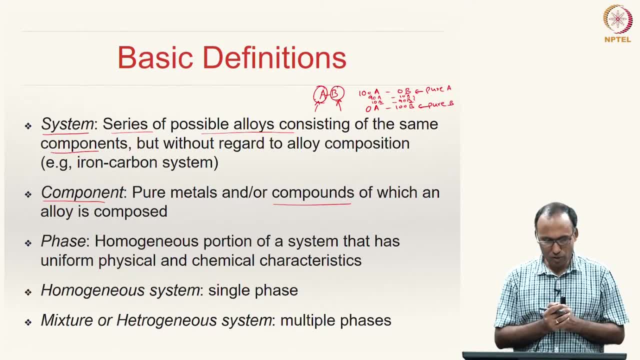 compound, another can be a pure metal, And so on. So if you are making an alloy out of these things, so these pure metal or compounds are called components, So for instance your solvent and solute, for instance, if 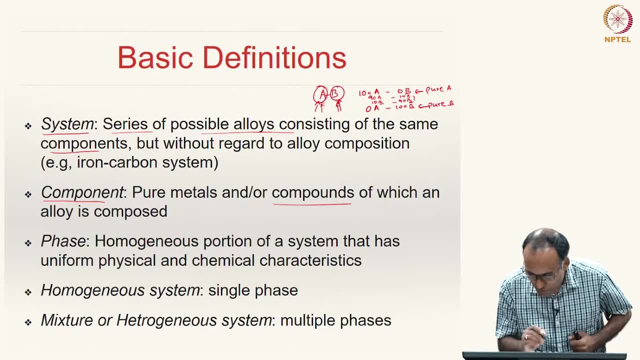 you take a two component system. So if you take A and B, there are only two components in alloy there are. such a system is called binary system And in this class we will only be dealing with binary system. And what do we mean by phase? A phase is nothing but the way that the phase should be defined. 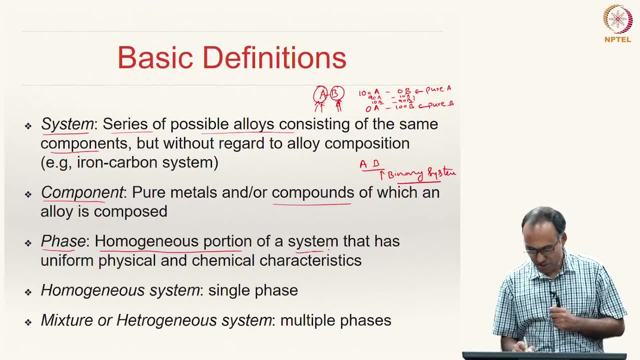 is the homogeneous portion of a system that has uniform physical and chemical characteristics. A phase is nothing but a homogeneous portion of a system that has uniform physical and chemical characteristics. that is what we call a phase. So suppose, if you take a solution of A and B, 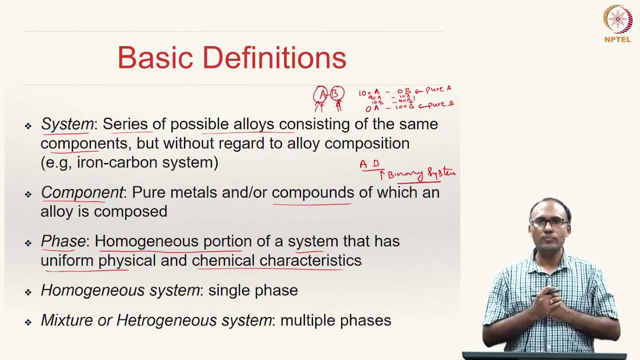 In the liquid state. it has certain properties, uniform physical and chemical characteristics in the liquid state, and hence it is called liquid phase. If it is coming in the solid phase and if it has uniform physical and chemical properties, then that is called another phase. 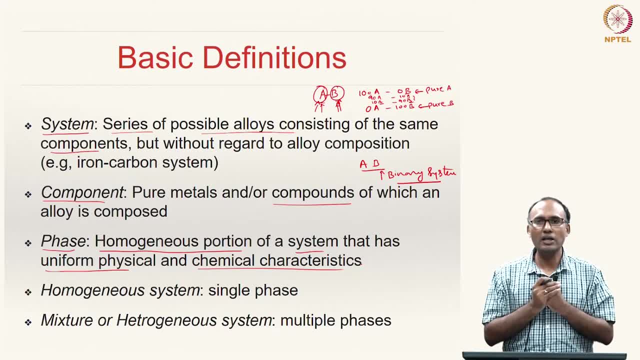 And you can actually have multiple phases in a liquid state or a solid state, And we will see. that means when we say multiple phases, each phase has a specific kind of physical and chemical properties. And what do we mean by homogeneous system? Homogeneous system is nothing but system which. 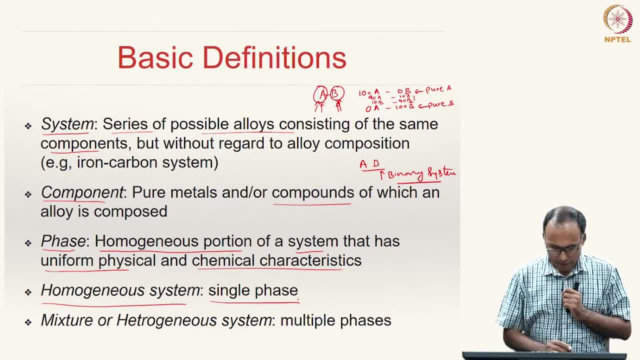 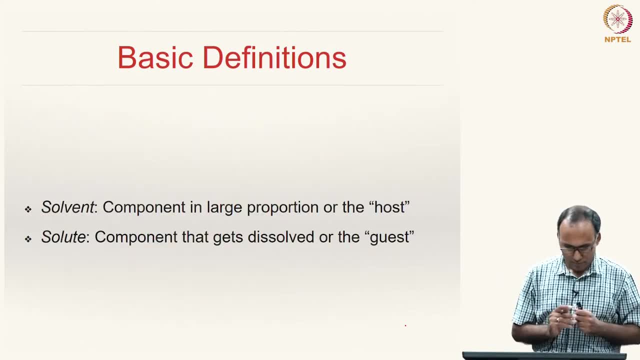 has only a single phase, And mixture or heterogeneous system is the one which has multiple phases. And we know already the definition of solvent and solute. we have already looked at it in the previous classes. So solvent is the component in larger portion or the host, and solute is 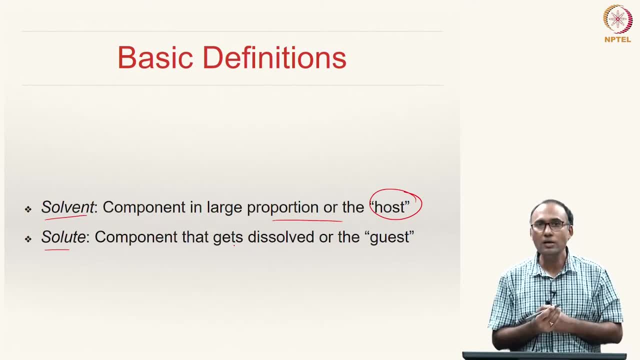 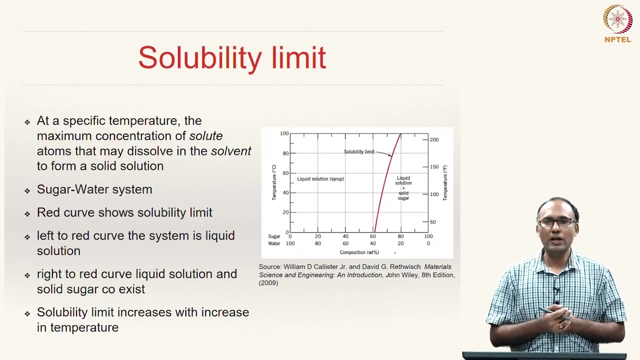 So solute is the component that gets dissolved in the solvent, or component can- sorry, solute can be thought of as guest, which is actually coming and sitting amongst the solvent cloud or host cloud. all right, So next we will try to understand the important concept called solubility limit. 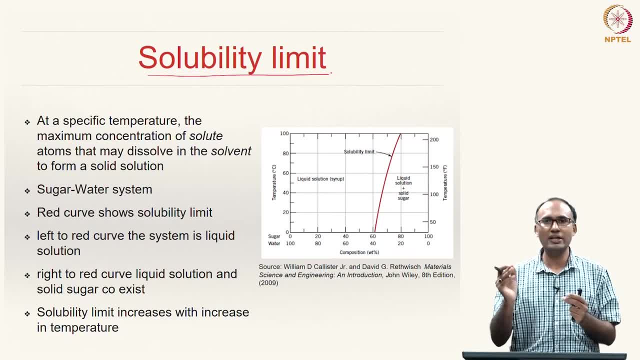 As we have discussed, there is a limit to which you can add a material A to material B and vice versa, and that is what we call a solubility limit. So, at a specific temperature, the maximum concentration of solute atoms. What is the maximum concentration of solute atoms that can be dissolved in the solvent? 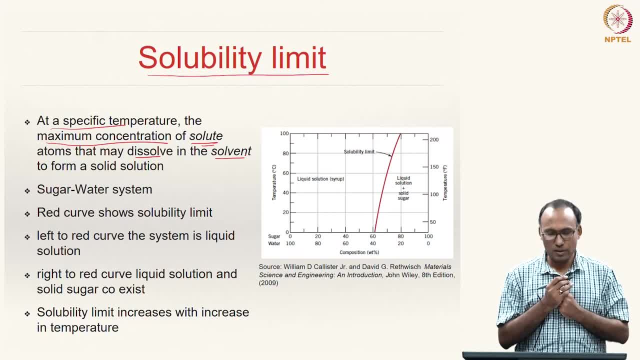 to form a solid solution and that is what you call solubility limit. So the maximum concentration of solute atoms that can be dissolved in the solvent to form a solid solution is called solid solubility limit, For instance. For instance, we can take the example of sugar water system here on in this graph, the red 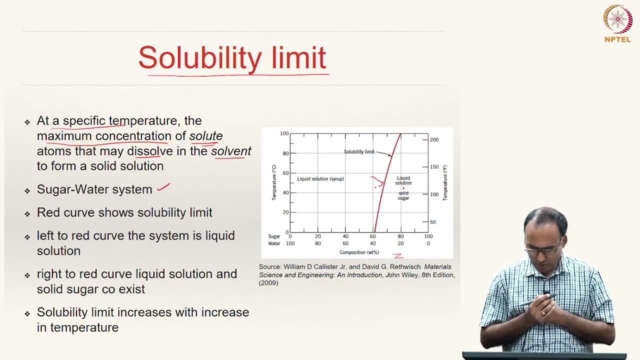 curve here. this curve here shows the solubility limit of sugar water system. So the left to right. So here we are seeing the temperature on the y axis and the x axis you have composition. So left to this red curve. 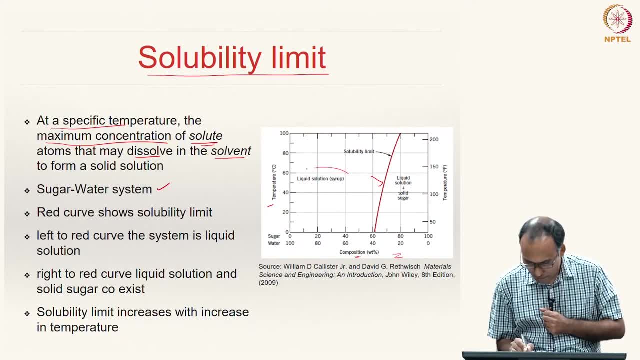 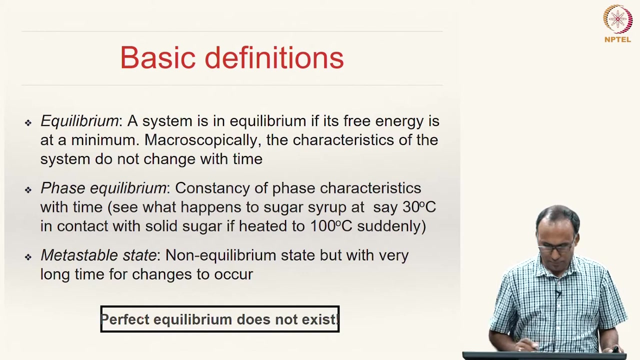 See this left to this regulation. there is an increase with increase in temperature versus this sugar water. And what do we mean by equilibrium? So when we say a system is in equilibrium, if its free energy is at a minimum, then free. 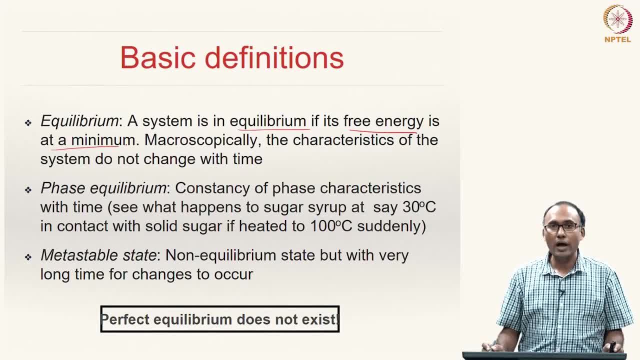 energy of the system should be at a minimum and microscopically. when some system is at equilibrium, the characteristics of the system do not change with time. that is the key equilibrium as a function of time, if you, if you are seeing that component today and come. 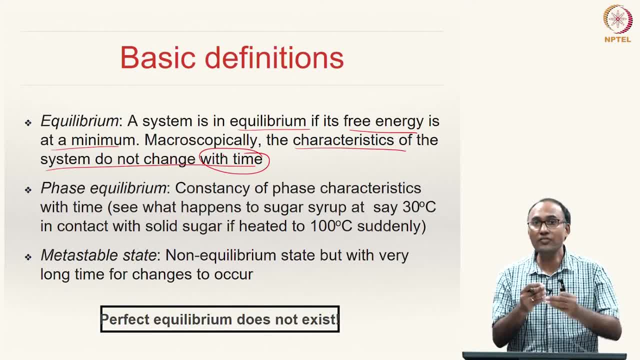 back after 100 years, it will still remain the same if it is in equilibrium state. ok, So the characteristics of the system should not change with respect to time, and such a such a configuration is called equilibrium configuration, or such a system is called is said to be in equilibrium. And what do we mean by phase equilibrium? Phase equilibrium: 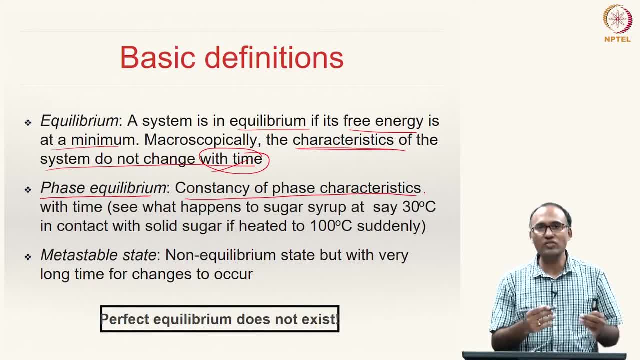 is nothing but the constancy of phase characteristics, as we have seen there are in the liquid sugar water solution. you have in the liquid state. you have liquid solution in the solid state. you have two phases: liquid phase as well as solid phase. The constancy of phase characteristics. 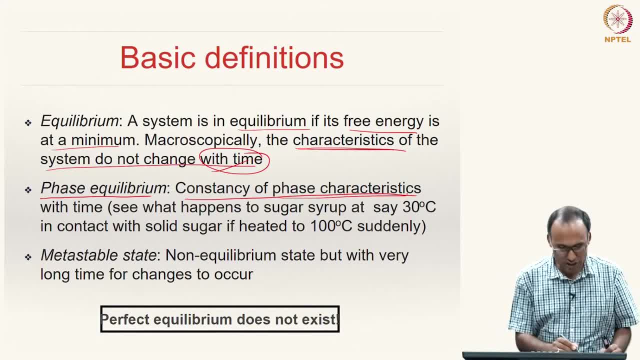 that means the characteristics of the phases should remain constant with time. ok, But at a at a given temperature. but if you are increasing the temperature, So for instance if you increase the temperature of sugar syrup, say at 30 degree Celsius in contact with solid, 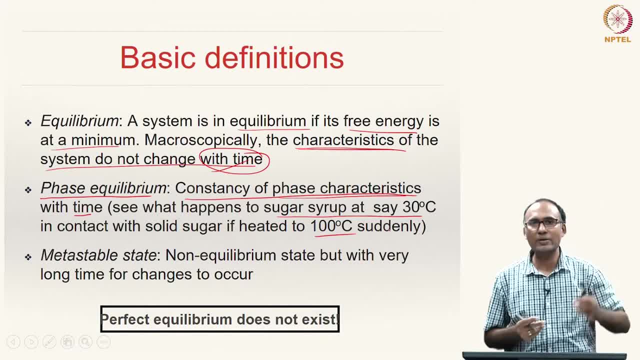 sugar. if you heat it to 100 degree Celsius, suddenly what happens? the solubility limit increases, and then the phases do not remain the same. the phases change with respect to time, And then it is when, then, we say that the phases are not in equilibrium, because 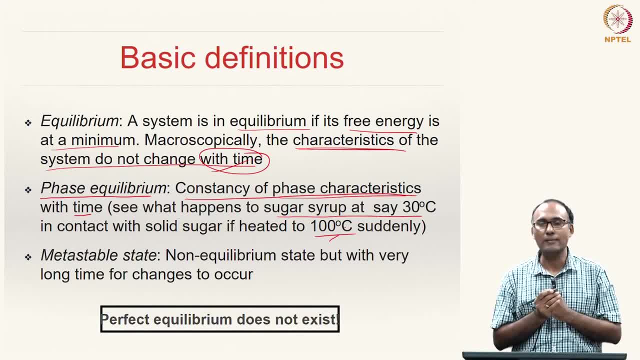 they are changing with respect to time when we are increasing the temperature. suddenly, ok, And then very important state called metastable state. what do we mean by metastable state? it is actually a non-equilibrium state, but with very long time for changes to occur. that 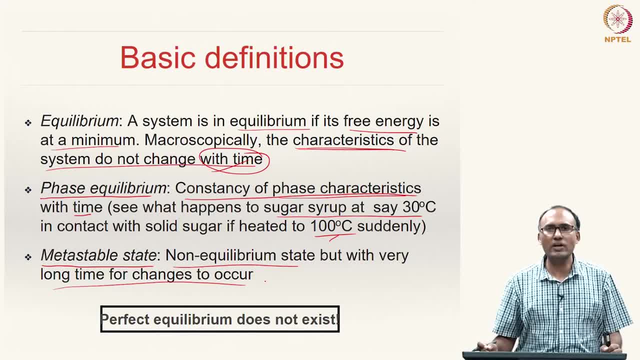 means it takes sufficiently long time for changes to occur. For instance, if you take an iron rod and leave it in open atmosphere, why may be? in one or two days? if you come back and see, you may not observe a significant change. But if you come back and see, maybe say a month a go, a month after or a year after, then 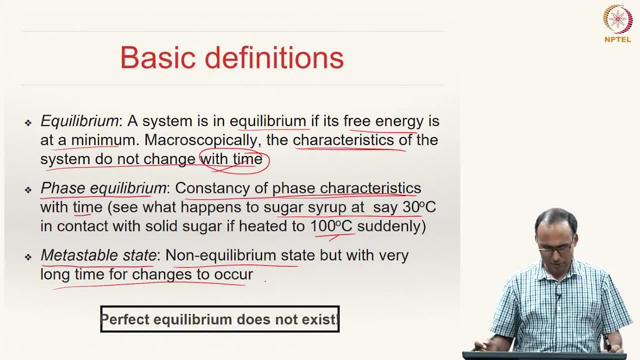 you will see that the iron is actually getting rusted. That means there is something, some change is happening to the phases that are present in the system, because of which the iron is rusting, And hence, but this change is happening over a long period of time. it is not happening over a short period of time, And hence such 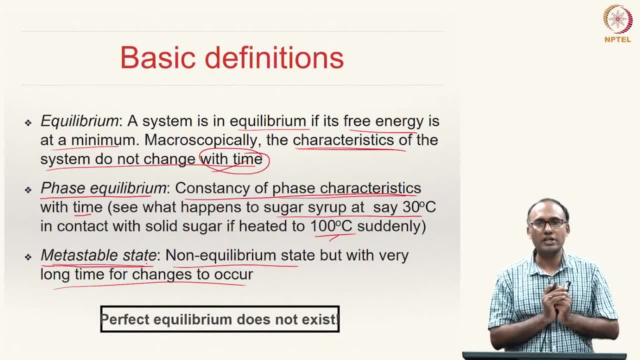 a state is called metastable state, So it is a non equilibrium state, but the changes are happening over a long period of time And please note that for any system that we are, for any alloy system that we will be discussing, the perfect equilibrium does not exist. So 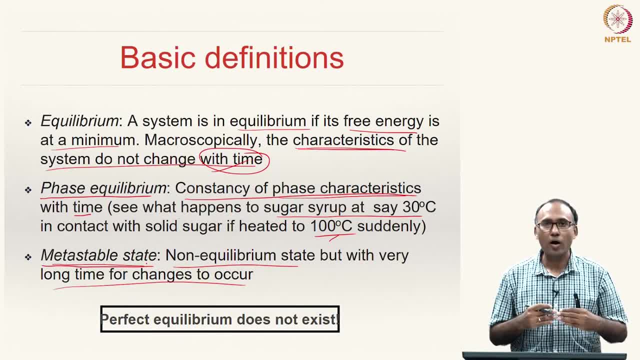 all the equilibriums that we are we are mentioning are usually metastable states because over a long period of time. that long period may be few hundred years, sometimes, right, but nevertheless, even after few hundred years, there may be some change in the phases, right. 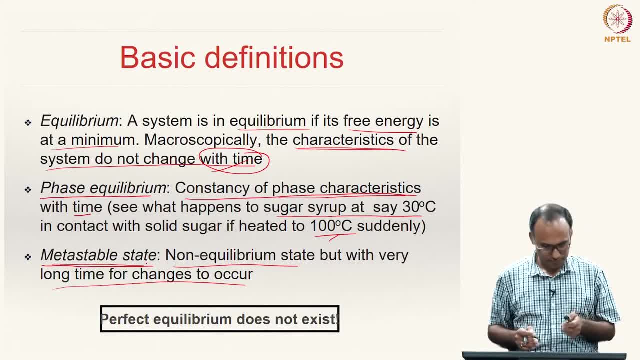 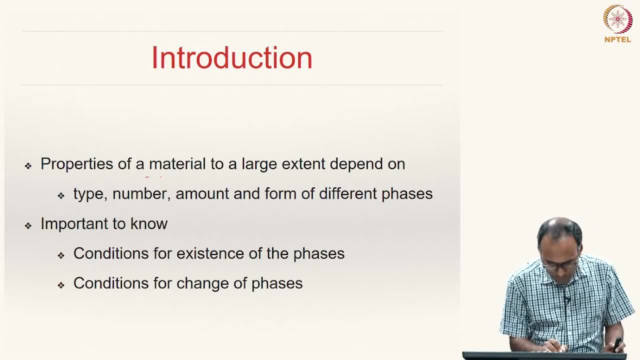 And such a state is what we call metastable state. And we know that the properties of a material or an alloy in this case, as we have discussed so far, to a large extent depend on The type, number, amount and form of different phases, what type of phase it is, how many. 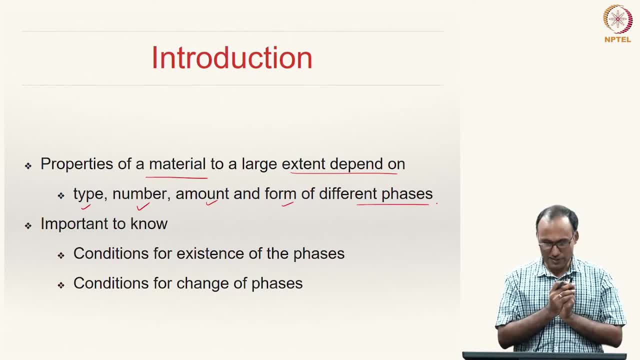 phases are there, what is the weight fraction of each and every phase and what is the micro structure of these phases? ok, All these determine the properties of the material. ok, And it is important to know the condition for existence of these phases. So suppose, let us say, a particular. 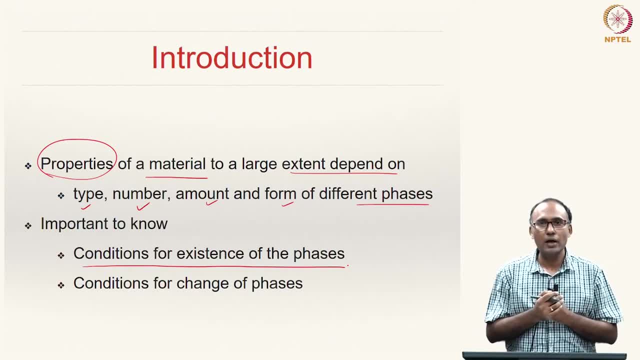 phase is going to give you an desirable property, and one there as an engineer. we should know what are the conditions under which such phases become a reality- that means they become viable or they exist- And what are the conditions for change of phases. so you got some phase. 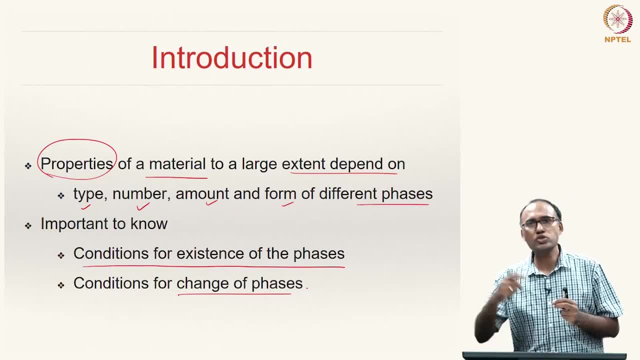 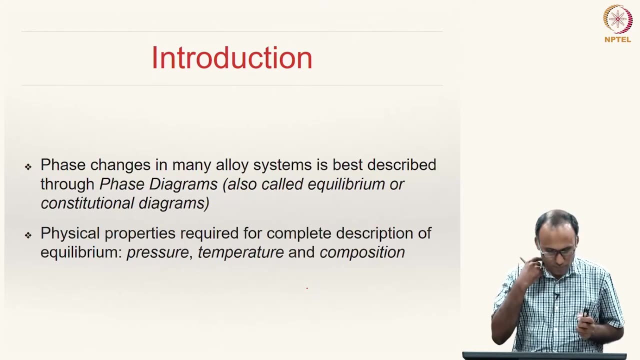 and what are the conditions under which the particular phase changes to some other phase. So this information is something that one needs to know in order to be able to use in the alloys with the utmost efficiency, as we know. So the phase changes in many alloy. 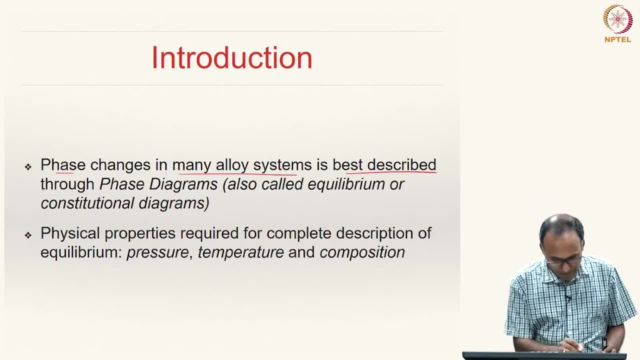 systems is best described by phase diagrams. The phase diagrams are also called equilibrium diagrams or constitutional diagrams. they are synonyms. The phase changes that we are discussing- we have posed the questions question in the previous slide. what are the how the changes occur? and the answer to that is usually given by understanding the phase diagrams, or phase. 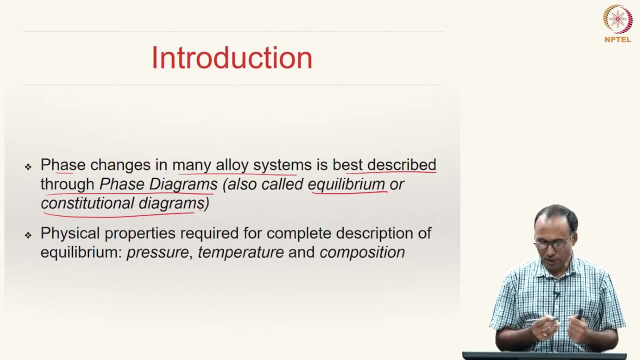 diagrams give answers to the question on how the changes occur, or from one phase to another phase, and are what conditions And the physical properties required for complete description of equilibrium phases are the following: They are pressure, temperature and composition. So these the phases that we are discussing. 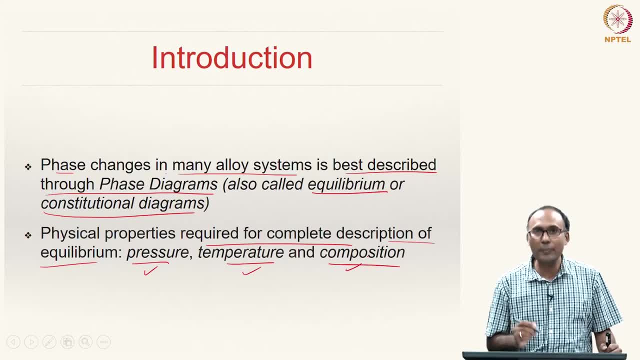 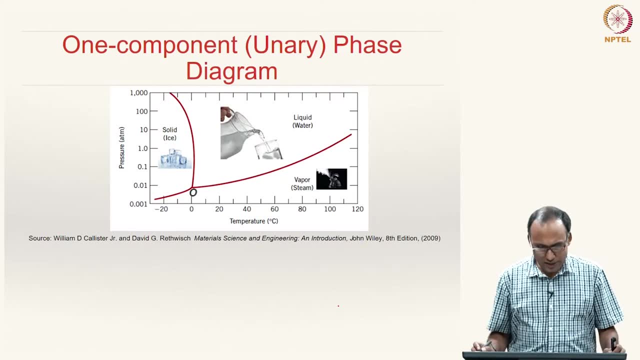 in an alloy system depends on these three independent variables: pressure, temperature and composition. So now let us look at, for the sake of understanding, a unary phase diagram or one component phase diagram. So that means there is only one component. that is what the 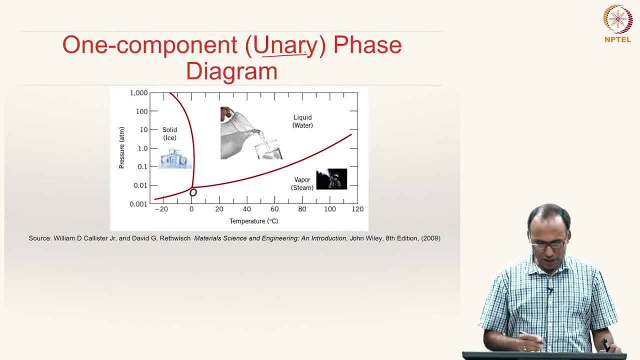 is that is known as unary phase diagram. Here we are looking at the phase diagram of water. So here we are having, because it is a unary phase diagram, the composition does not come into picture, and the composition comes into picture when there is more than one component. 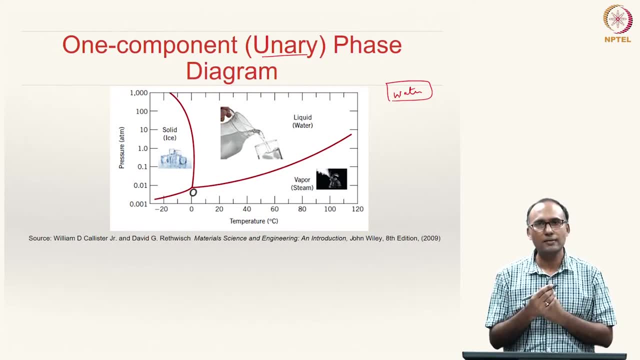 right, because there is only one component. it will be there 100 percent. So the composition does not come in picture, and hence the other two variables are pressure and temperature. So here on the y axis, we have pressure on the y axis, we have pressure on the y axis. 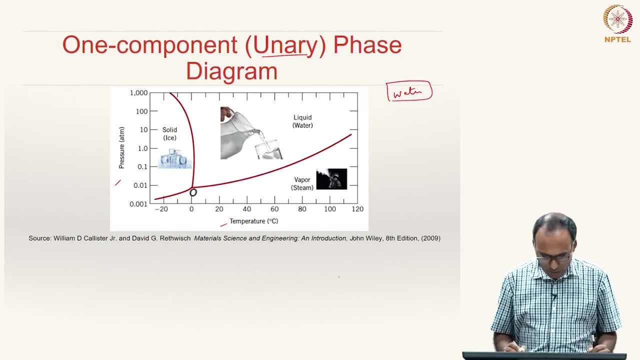 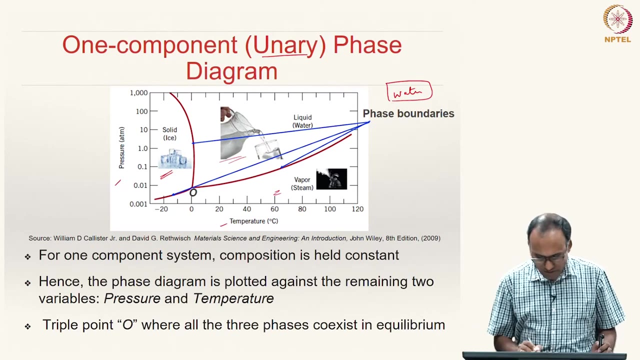 on the x axis we have temperature in degree Celsius And these, the boundaries that shown in the reds, are called phase boundaries. and here, on this region, you have liquid water, solid ice and this is vapor region. So for one component system, the composition is held constant because there is no variation of component, and hence the phase diagram is. 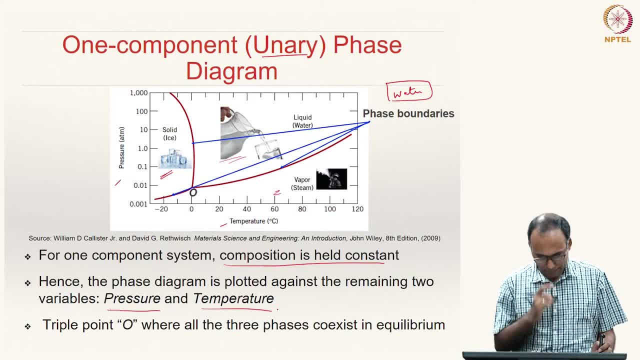 plotted against pressure versus temperature. And here you can see the triple point O and O surface, where all the three phases co-exist and all other boundaries the two phases co-exist. For instance, if you take this boundary, this: this is the boundary between solid phase and 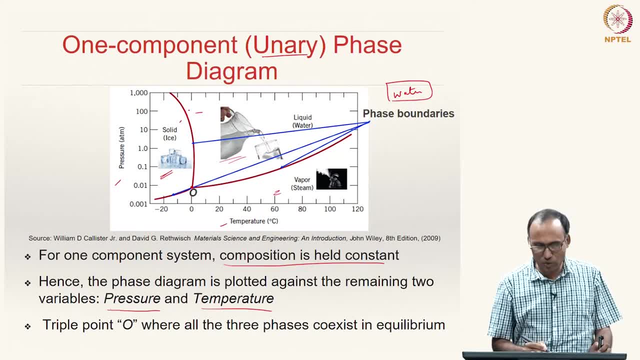 liquid phase And hence, on this boundary, both solid and liquid co-exist, and this is the boundary between solid and vapor, and hence solid and vapor coexist on this boundary. you have this boundary, you have liquid and vapor and hence these two on that, on that boundary for various temperatures and pressures. 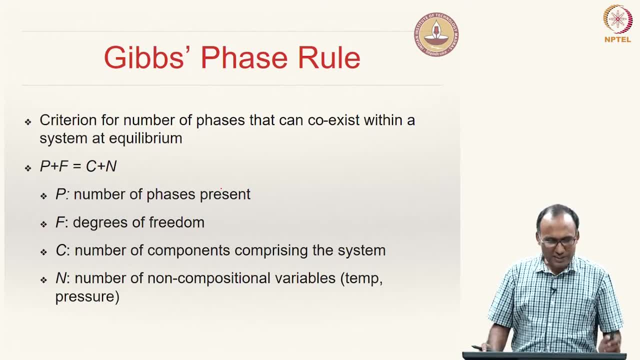 So now, what is the criterion for finding the number of phases that can coexist within a system at equilibrium? I am sure that all of you are familiar with this Gibbs phase rule, which says that p plus f equal to c plus n, where p represents the number of phases. 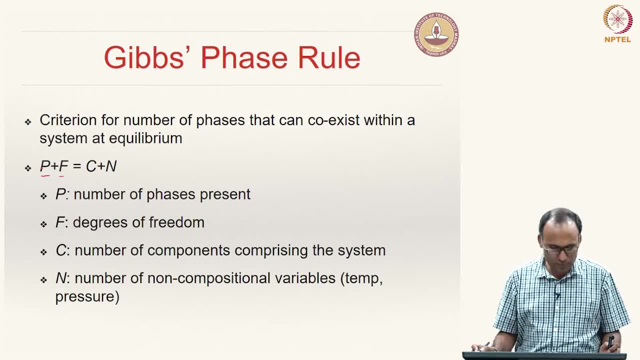 present. f represents the degrees of freedom c. we will see what we mean by degree of freedom. c is the number of components comprising the system. n is the number of non-compositional variables. Here non-compositional variables are temperature and pressure. So the number 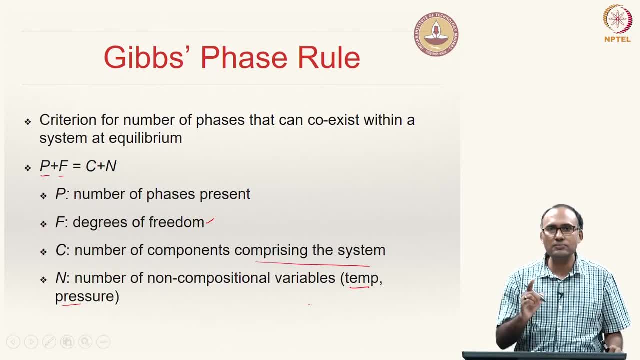 of components comprising the system. how many components are there? It is a unary phase diagram and hence c is equal to 1.. And now, the number of phases present at equilibrium is something that we will look at, and the number of compositional variables are 2, n. 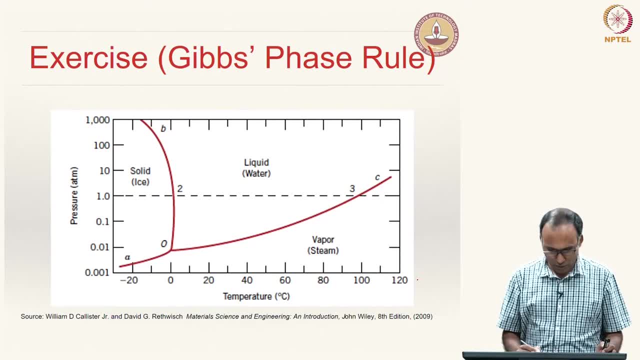 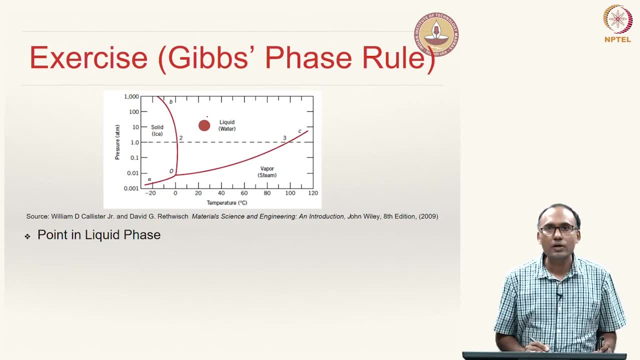 equal to 2.. So now let us look at it. If you are in the liquid phase, how many phases are present? only one phase, right, It is a liquid phase. So p equal to 1 and number of components equal to 1, n equal to 2, n is number of non-compositional variables. 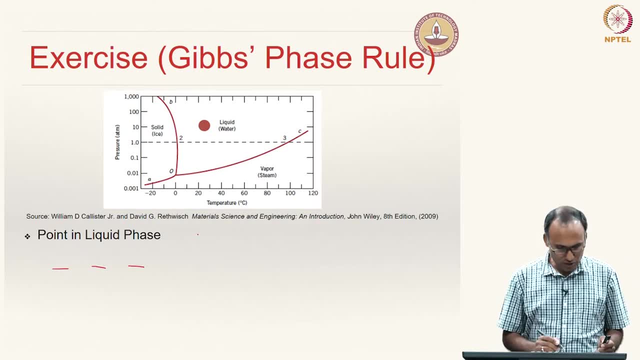 So we know that p plus f equal to c plus n. that is the number of non-compositional plus n, right, that is what we have written. So using that, f can be written as c plus n equal to 2.. So c plus 2 minus p, that equal to 2, which means we have a degree of freedom. 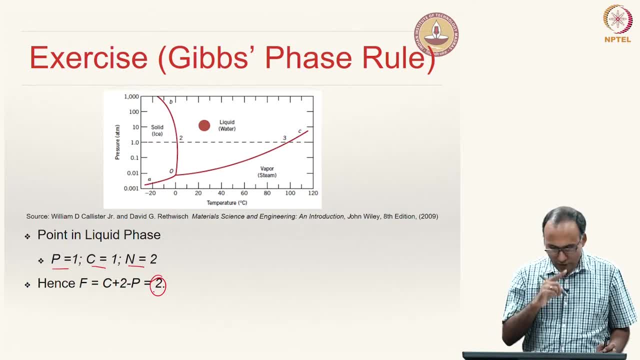 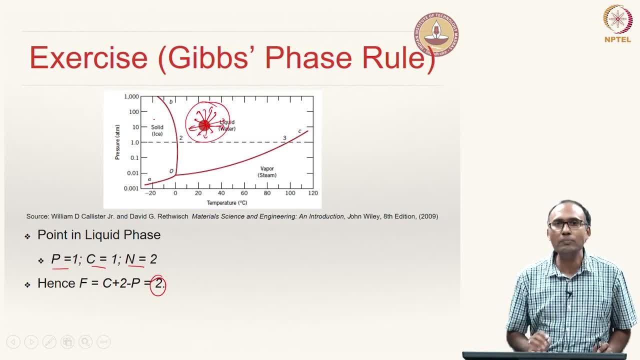 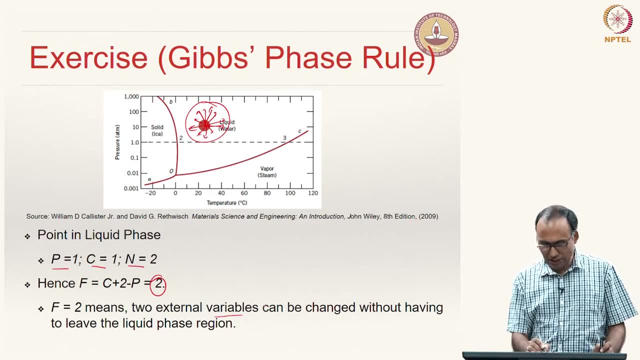 Even if you move, you will still remain in the same state. then the in the liquid phase only. that is what we mean by degree of freedom. So f equal to 2 means 2 external variables that are present. temperatures can be changed without having to leave the liquid phase region. 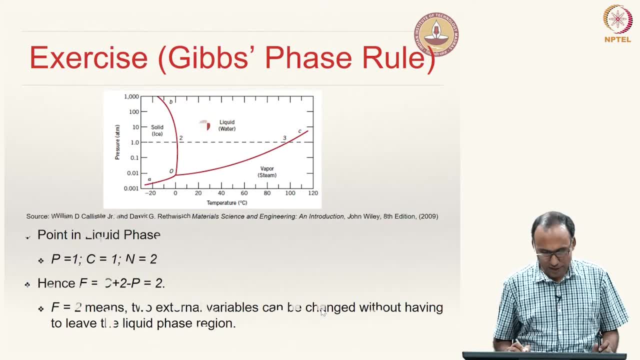 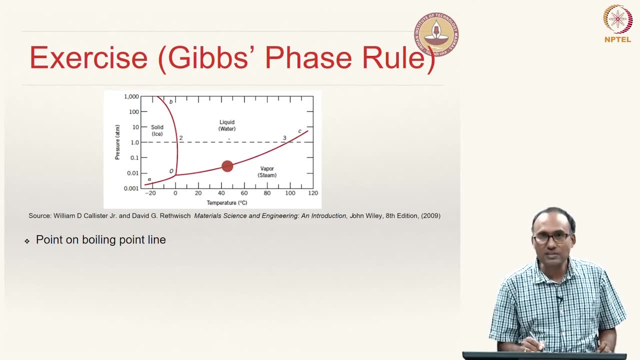 you will still be in the liquid phase. Now you are on the boiling point line, that is, liquid vapour interface. So, as we know that this is a two phase, on this line two phases coexist. What are the phases? The liquid- 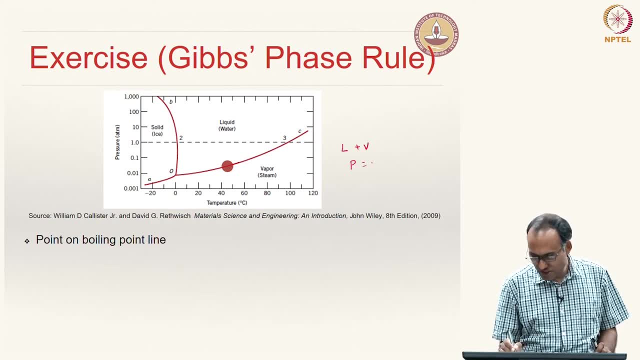 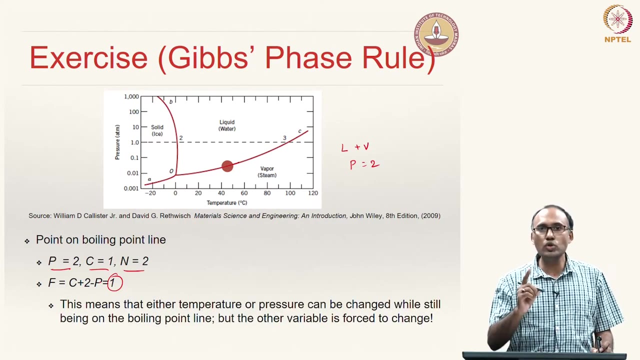 phase and vapour phase coexist, So the number of phases are 2, and c and n will be the same and, as a result, your f will become equal to 1.. What is the meaning of that? You have only freedom to choose one of the external variables to be chosen. So this: 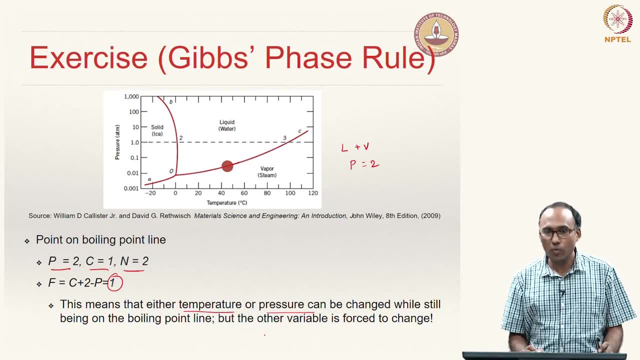 means that either temperature or pressure can be changed while still being on the boiling point line, but the other variable is forced to change to in its own way. That means you can only move this way, So you can choose what should be my temperature change and automatically. 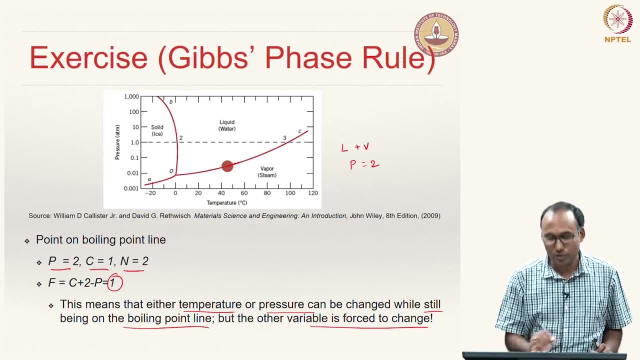 pressure change should be decided by this guy, Right this line. but if you want to move in any other way, then you will be leaving the two phase region, right. So that is, that is the degree of freedom 1. Now let us look. 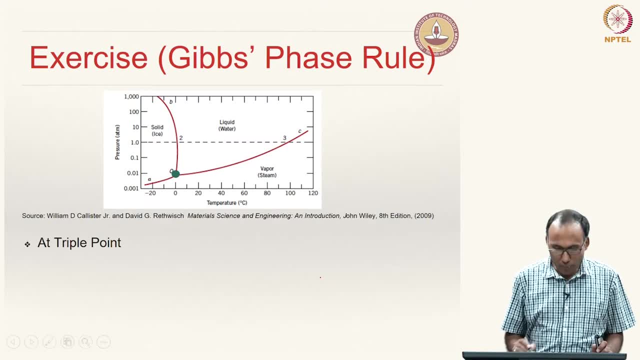 at the triple point. So how many phases coexist here? both solid, liquid and vapour? sorry, not all 3. solid, liquid and vapour: all 3 phases coexist at the triple point and hence number of phases present are 3.. 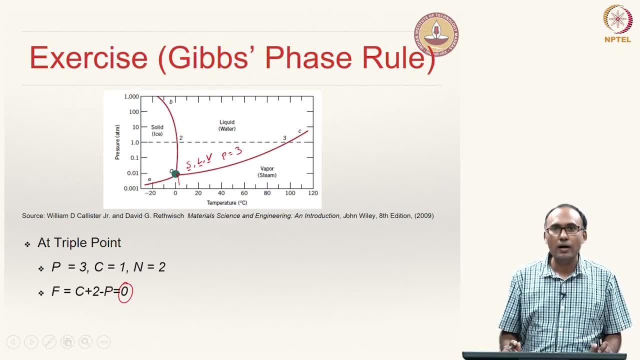 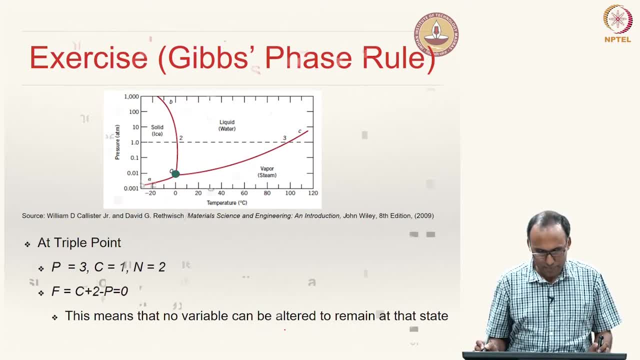 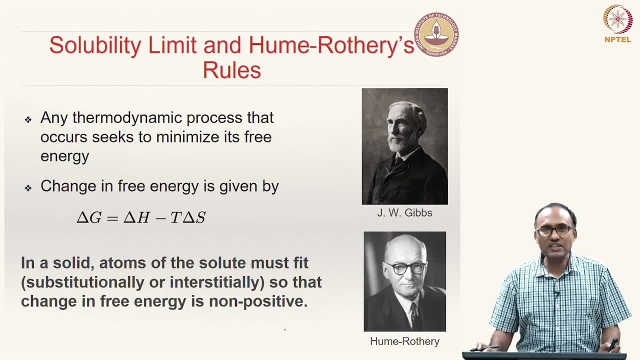 altered to remain at that state. all right, Now let us look at. we have discussed the solubility limit and there are certain rules put forth by Hume Rothery's- they are famously known as Hume Rothery's rules for the formation of solid solutions. 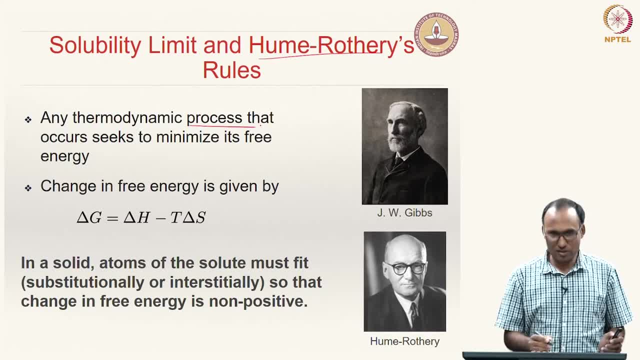 First of all, any thermodynamic process that occurs seeks to minimize its free energy. that is important. So the free energy can be written as: delta H minus change in free energy is equal to delta H minus T delta S. So if in a thermodynamic process the process should: 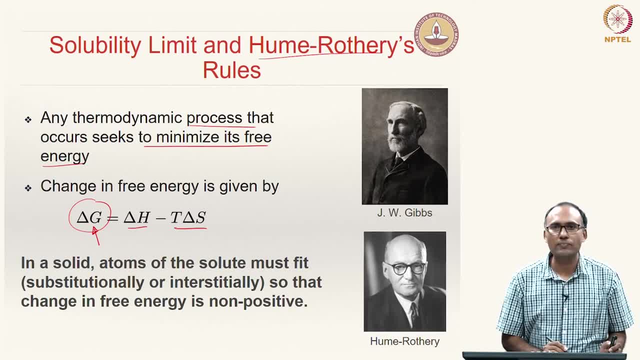 happen in such a way that this delta G is non negative. sorry, delta H minus T, delta S is G, is non positive. that means it should be negative only when delta G is negative. that is, when you are continuing to reduce your free energy, as we have discussed here. 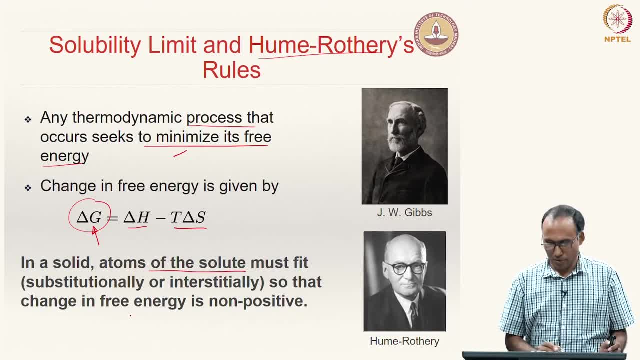 So in a solid atoms of the solute must fit either substitutionally or interstitially so that the change in free energy is non positive. this is the requirement when you are adding a solute atom to solvent atom And they will be non positive. So the change in free energy is non positive. this is the 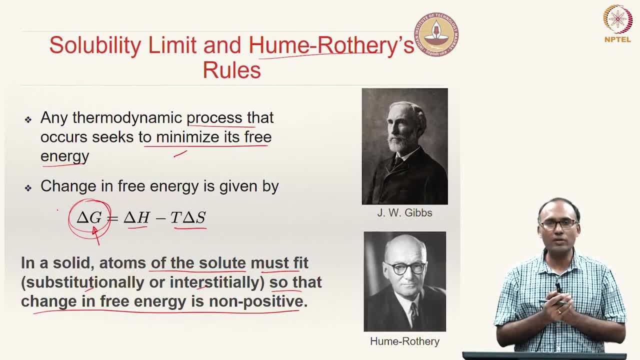 requirement when you are adding a solute atom to solvent atom, and they will be non positive, So they will. they should fit into the solvent cloud, but effectively resulting in net reduction in the free energy. only then such a thermodynamic process, thermodynamic process, is feasible. 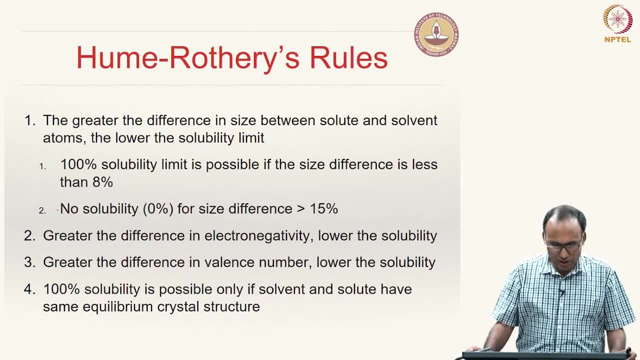 ok, So what are the Hume Rothery's rules? the greater the difference in size between solute and solvent atom, the lower the solubility. that means, if you want to have higher solubility- the for instance, for instance, If you are taking about talking about binary phase diagrams- if you want to have higher, 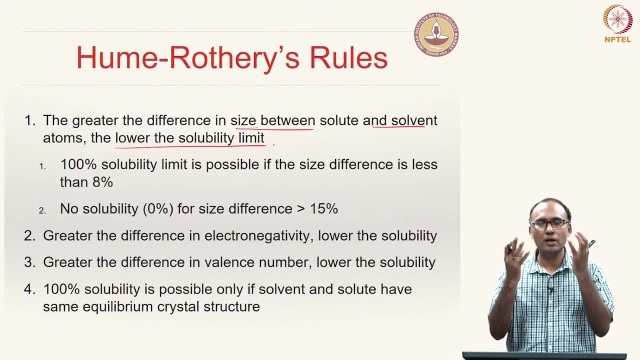 solubility, the size of both the components atoms, the solvent and solute atoms. sizes should be almost similar. there should not be huge size difference between them. So 100 percent solubility of A in B and B in A is possible if the size difference is. 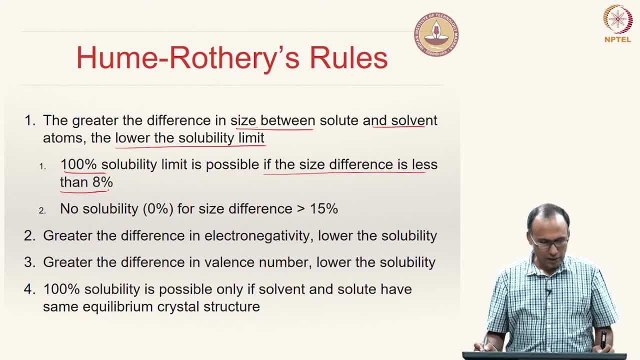 less than 8 percent, And If your size difference between atom A and atom B is greater than 15 percent, there is almost no solubility. if we said 0 percent, but it is almost no solubility, it will not so dissolve in that suppose if the difference between A and B is greater than 15 percent. 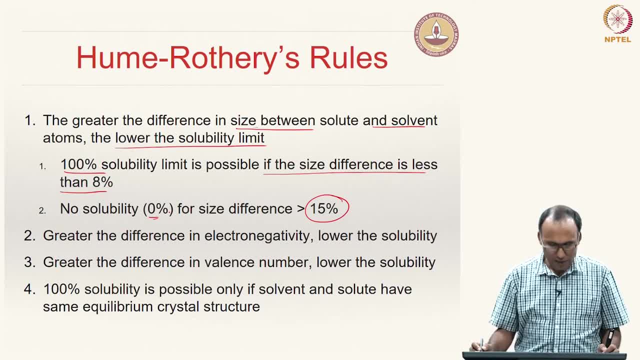 then the materials do not get dissolved for them to make a substitution of solid solution. the reasons, the rules that we are talking about here are true for substitution of solid solutions. So numbers may be very different, little different for interstitial solid solutions. So, but here we are focusing on substitution of solid solutions, just to get an idea. 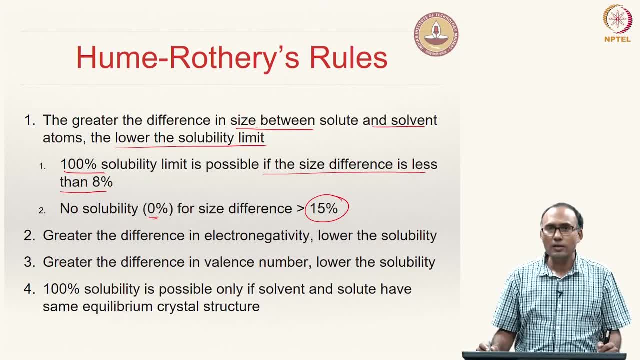 And again, the solubility is will diminish if the electronegativity values of these two atoms are very different. So if you want to enhance the solubility, there should be their electronegativity values also should be very close to each other. 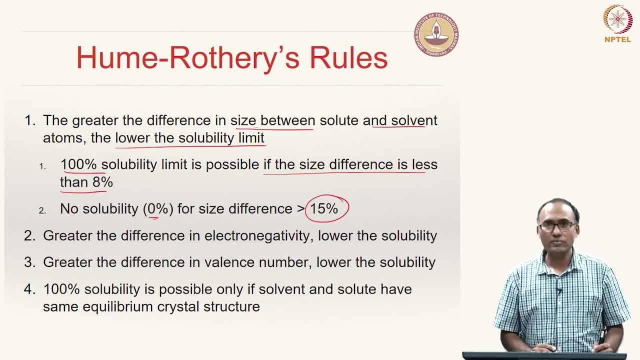 And The Valence number. The difference in valence number should also be very close, should be very less. That means the valence number of atom A and atom B should be as close as possible in order to have greater solubility. 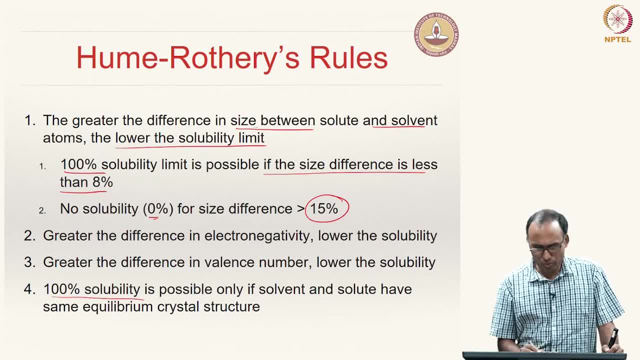 And 100 percent solubility is possible only if solvent and solute have same equilibrium crystal structure. that is another important thing. If a solvent atom is A is FCC and solute should also be FCC, only then you will have 100 percent, 100 percent solubility. otherwise 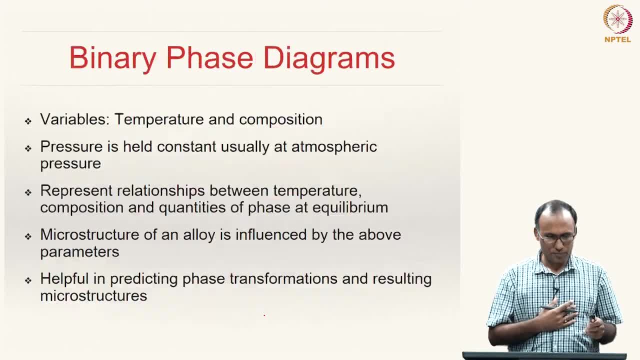 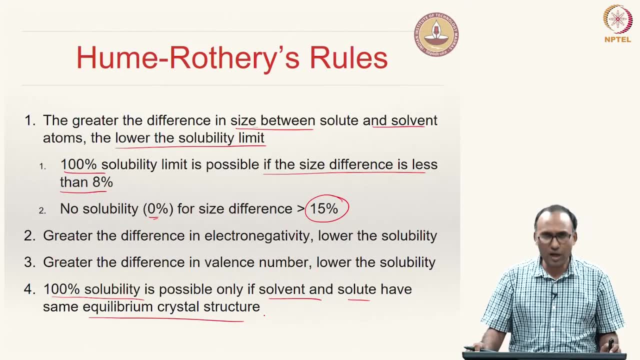 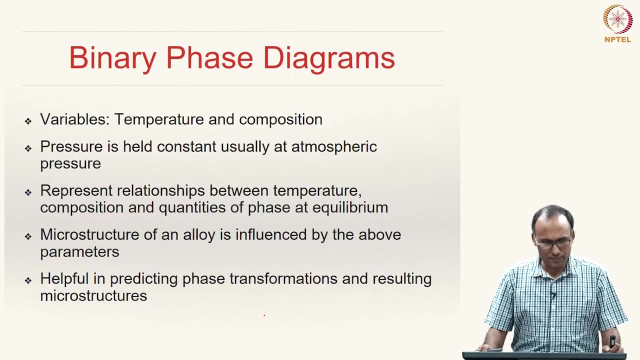 you will not have 100 percent solubility. So this Hume-Rothery's rules that we have discussed here are primarily suggested, based on observations, and these four rules that we have written are valid for all the substitutional solids. So now let us look at the binary phase diagrams, as we have discussed. when we say binary phase, 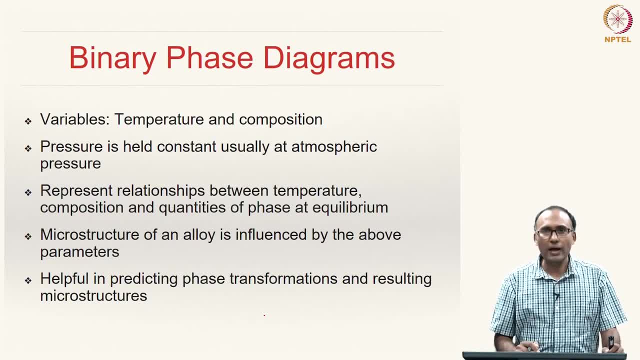 diagrams, you have two components, A and B, And here, as we have discussed, for describing a phase diagram, you will have three variables, three independent variables. what are they? pressure, temperature and composition. So, in this course, when we are drawing, when we are talking about binary phase diagrams, 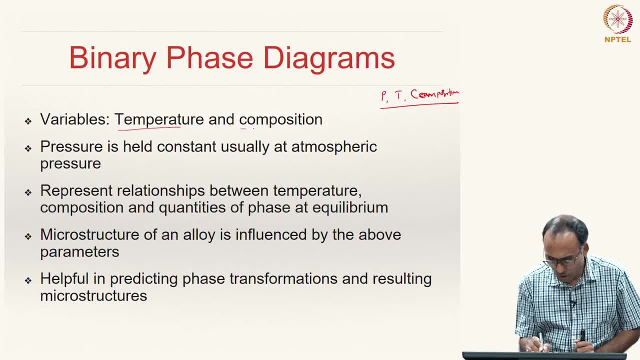 the two independent variables that we are choosing are temperature and composition, and typically that is how it is done for most of the phase diagrams, and pressure is usually held constant at atmospheric pressure. So all the most of the phase diagram that you would see in the literature are drawn with composition versus temperature by at one atmospheric 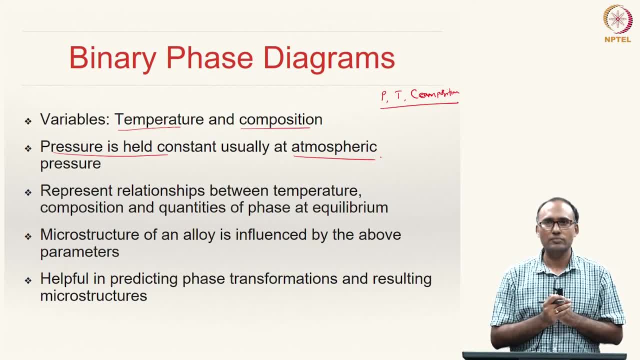 pressure And if there is a change in atmospheric pressure- sorry, when there is change in pressure other than atmospheric pressure- then the phase diagram will change when you are drawing between temperature and composition. But most of the phase diagram that we will be discussing- not all the phase diagram that we will be discussing in this class- are done at atmospheric. 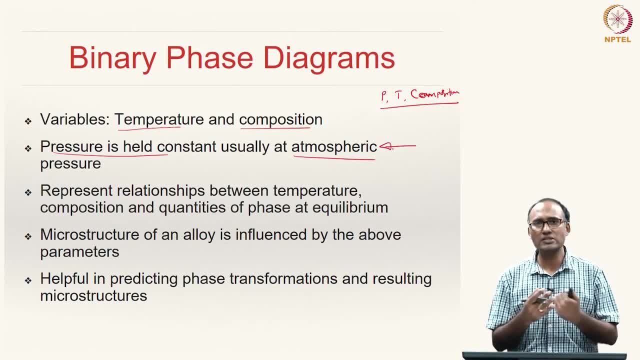 pressure, And that is also true for several phase diagrams that you would come across in the literature. So the binary phase diagrams represent the relationships between the temperature, composition and quantities of phases at equilibrium. What are the different quantities of, what are the different phases and what are their quantities? 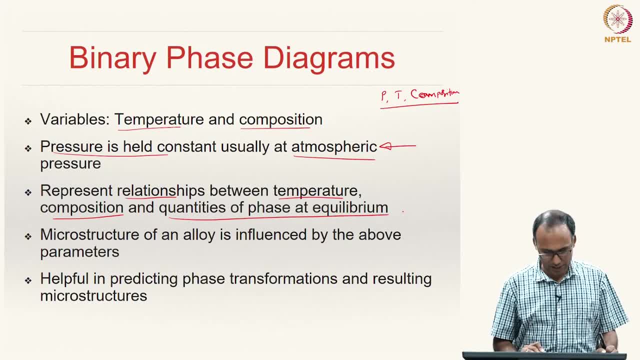 This is something that will be clearly described by a binary phase diagram. And note that the microstructure, the underlying microstructure of an alloy, is significantly influenced by the above parameters, particularly the composition and the temperature. These two guys are going to significantly influence the microstructure. So the binary phase diagrams help us in predicting. 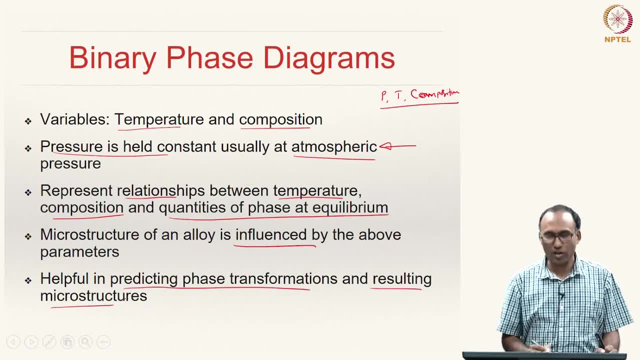 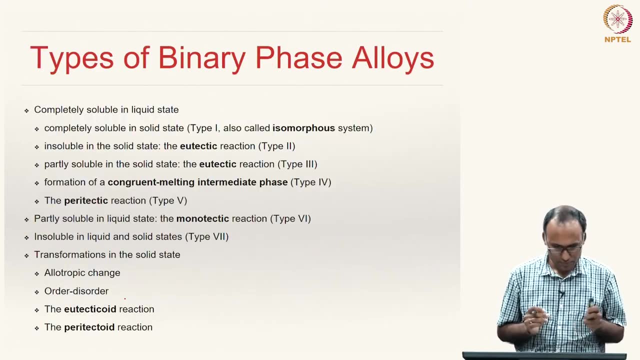 phase transformations and the resulting microstructures, How a particular phase transform to another phase and the resulting microstructure, Microstructure from through this phase transformations is something that we will understand through binary phase diagrams. So in this module, in this course, we will be discussing different. 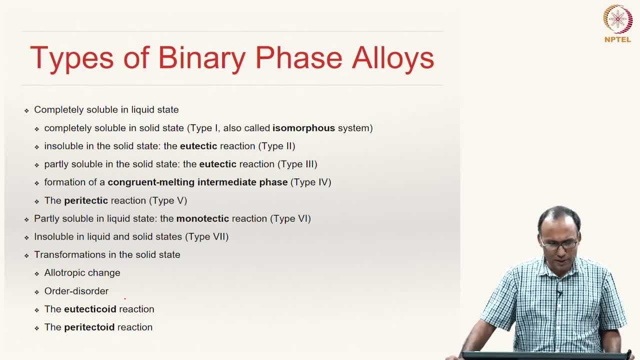 types of binary phase alloys. So here we have made a classification. So let us say you have alloy A or metal A and metal B. We are only talking about metallic alloys, So metal A and metal B. and if the first classification is that if metal A and metal B are soluble, 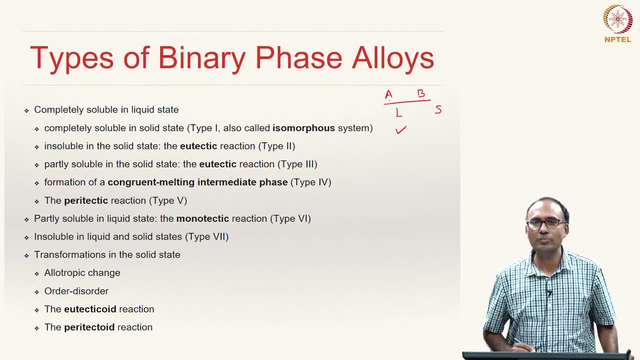 in liquid state. completely soluble in liquid state, That means there is 100 percent solubility possible in possible for A in B and B in A. When is that possible? When some of the rules that we have discussed. So the primary classification is that when we are saying that they are completely soluble. 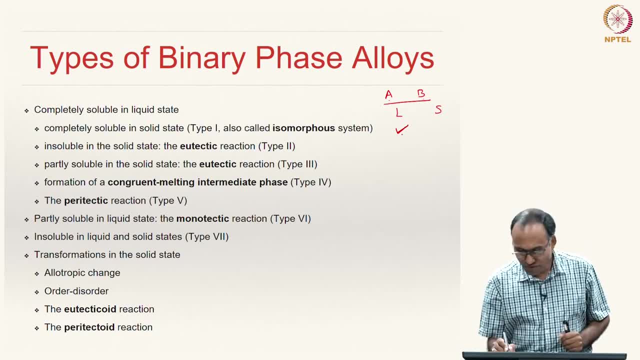 in liquid state, So of the materials that are completely soluble in liquid state. now the first type of alloys that we are going to discuss are called isomorphous alloys, which are also completely soluble in solid state. So isomorphous system is a system. 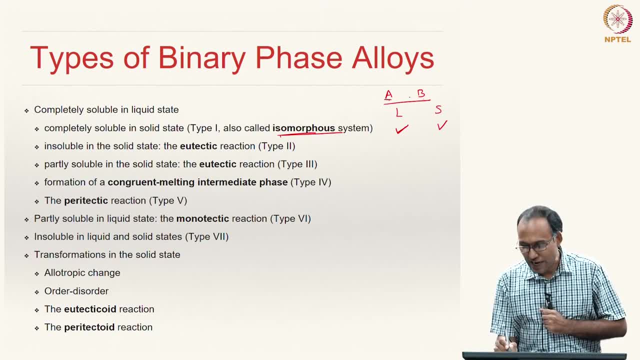 of alloys in which components A and B are completely soluble in liquid state and completely soluble in solid state. That means A is soluble in B and B is soluble in A completely, And then type 2, in type 2, we will look at a system wherein there is complete solubility. 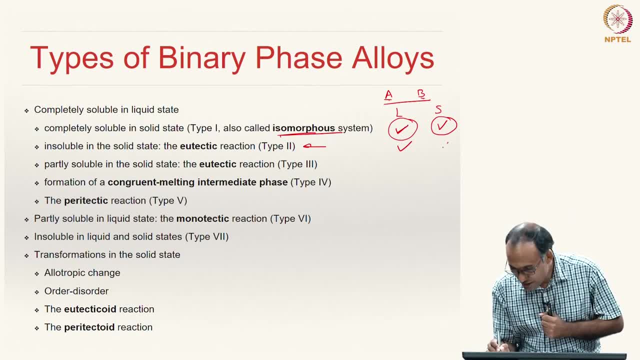 in liquid state, but there is no solubility in solid state. So there is no solubility in solid state, And when we are discussing this type of a system, we will look at a specific important reaction called eutectic reaction, or we will also discuss something called this. 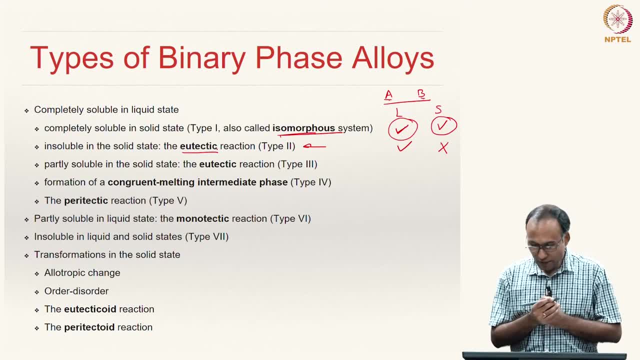 type of alloys are called eutectic alloys, And now the third one is somewhere in between these two. You have complete solubility in liquid state: 2., 3., 4., 5., 6., 7.. 8., 9., 10., 11., 12., 13., 14., 15., 16., 16., 17., 18., 19., 20., 21., 22., 22.. 23., 24., 25., 26., 27., 28., 29., 30., 31., 31., 32., 32., 33., 34., 35., 36., 36.. 37., 38., 39., 39., 40., 41., 42., 42., 43., 43., 44., 44., 45., 45., 46., 46., 47.. 48., 49., 49., 50., 50., 51., 52., 53., 54., 55., 56., 57., 58., 59., 60., 61., 62.. 62., 63., 63., 64., 65., 66., 67., 68., 67., 68., 68., 69., 69., 70., 70., 71., 72.. 71., 72., 73., 73., 74., 74., 75., 76., 77., 78., 78., 79., 79., 80., 80., 81., 81.. 82., 82., 83., 84., 85., 86., 87., 86., 87., 88., 89., 90., 90.. 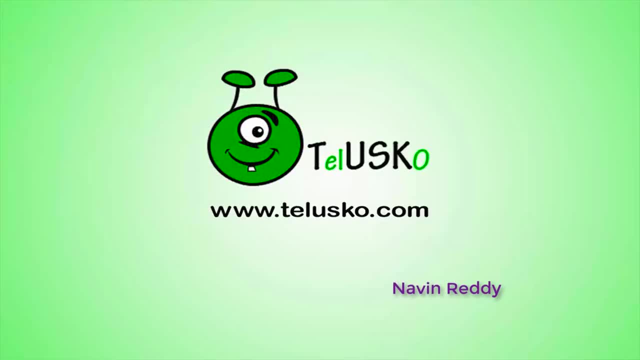 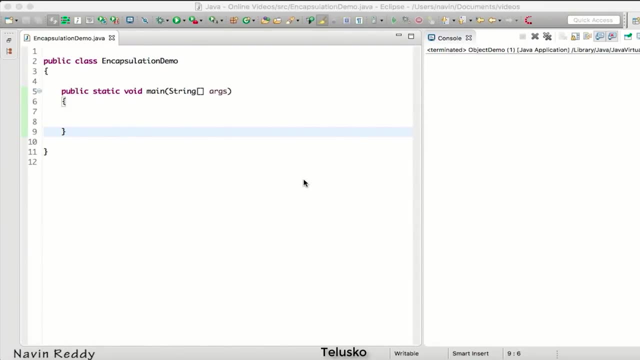 In this video we'll talk about encapsulation. So we'll divide the video into two parts. I mean not the videos, but the topic. In the first part of the video, we'll talk about what is encapsulation. In the second part of the video, we'll talk about why do we need it, So encapsulation. 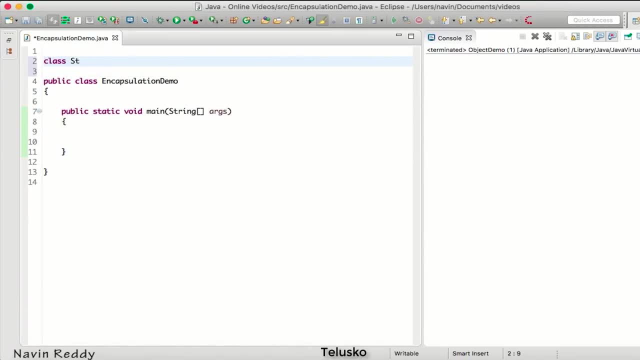 basically means is you'll be having a class and let's say this class is student In this class. normally what happens is class will. so object knows something. object does something right And we have done, we have seen that from a long time. So object knows something with the help of. 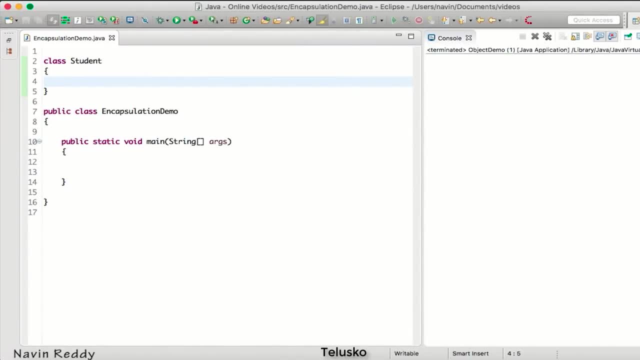 variables Object does something with the help of methods. So whenever you create any variable- let's say we have row number and we have name- we have to make sure that those variable data, so those variables, need to only be changed or fetched with the help of methods. So if you want, 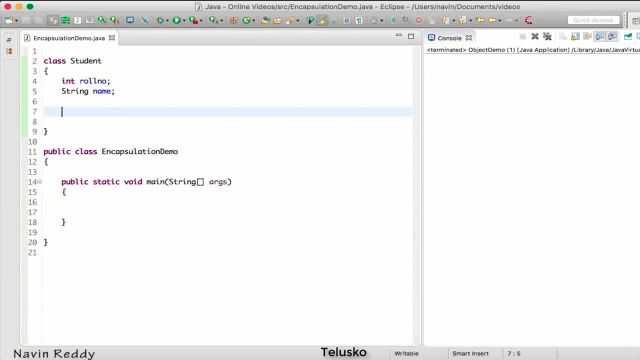 to do anything with the variables, you have to use methods. Okay Example: if you want to set the value of the row number, what we can normally do is we can create the object of student. We can say student S1, equal to new student, and we'll say S1 dot. row number is equal to two And we can say: